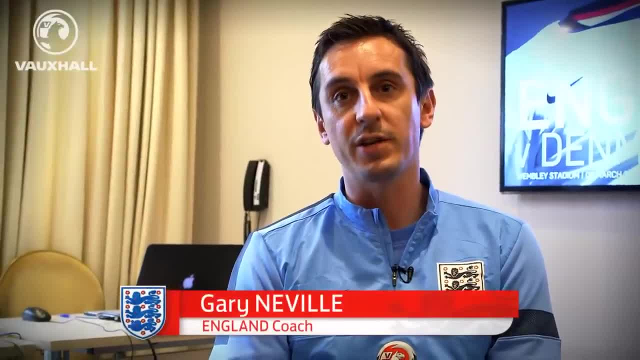 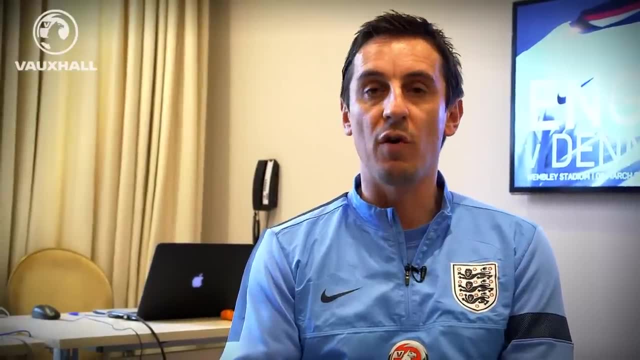 Yeah, it's very important- because obviously there's a restricted amount of training sessions- for the manager to be able to put his points across to the players. So this is another form, that is non-physical, of being able to give the players information and allow them. 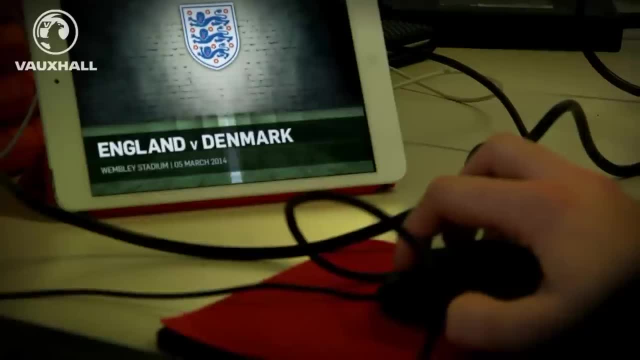 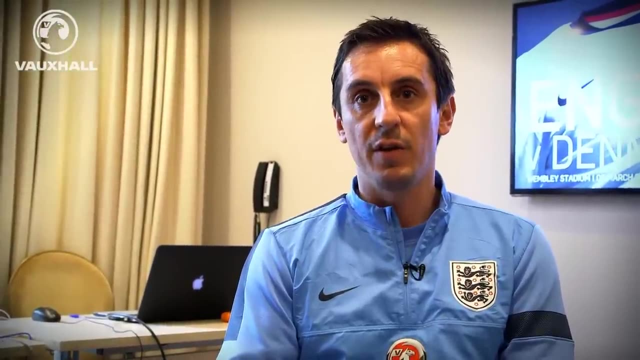 to know about the opposition, things that obviously are expected of the players themselves And, like I say, it's important that, like this time of the season in particular, that it's as important really as training sessions. we treat it as a training session. 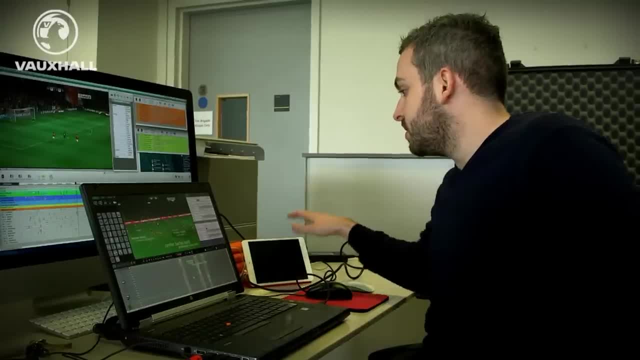 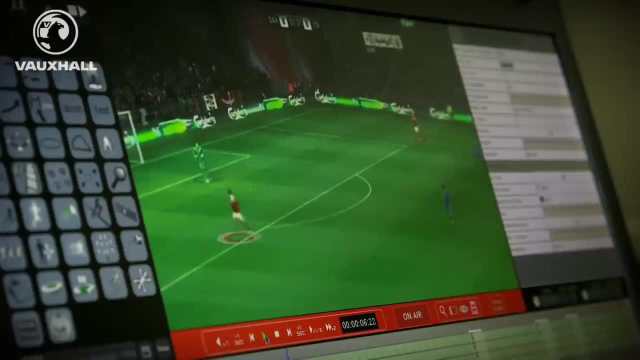 So when we meet up, they'll be given the iPads. they've all got their own iPad and everything will be on there, ready for them as soon as we get together. I think that the primary thing is always concentrating on our own strengths and weaknesses, but you 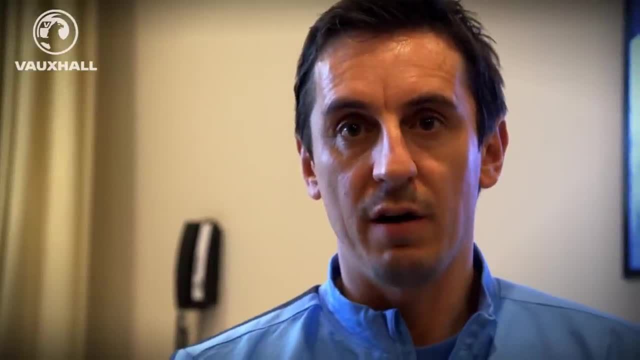 have to deal and pay attention to the opposition. It's an obvious part of international football and football generally now and I think that the amount of data that we get, given the amount of analysis we get, given it's an obvious part of international football and football generally now and I think that the amount of data that we get, given the amount of analysis, 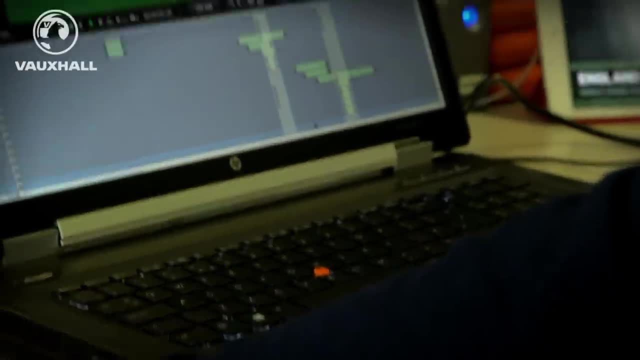 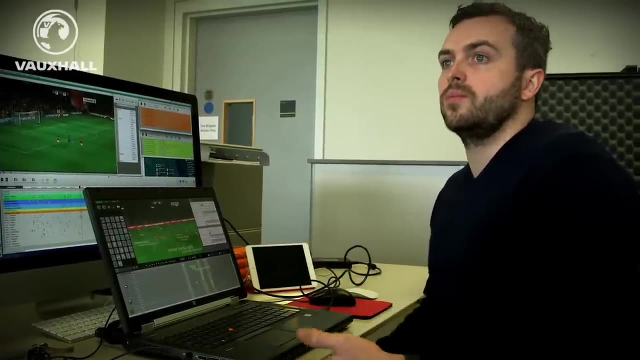 that goes on behind the scenes is incredible. now in football, and obviously it's the same here with England- Everything is on for everyone because the units interact with each other. What I put on for the right-back, he's going to need to see what their opposition left midfield. 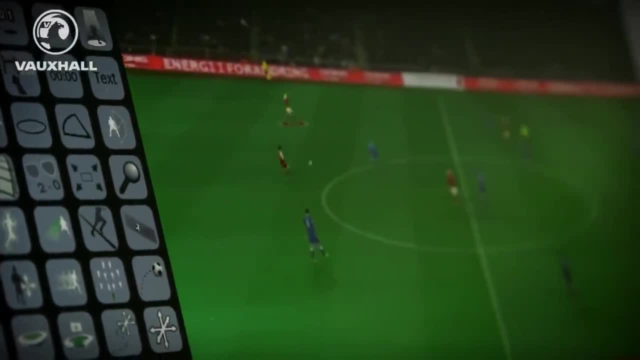 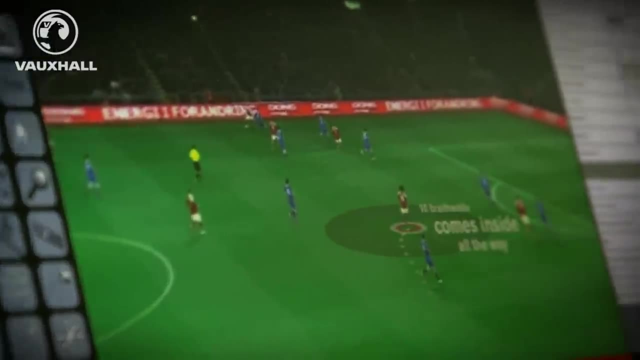 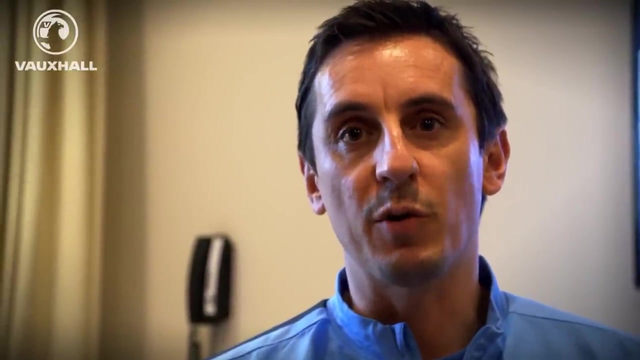 is doing what their opposition central midfield is doing, So they need to see everything. A centre-forward will make runs into areas where they will be, so they get everything the same as everyone else. You've got to be as compact as you can because you don't want to fill them with too much. 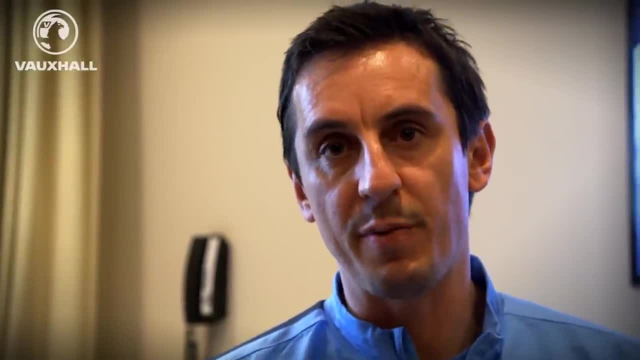 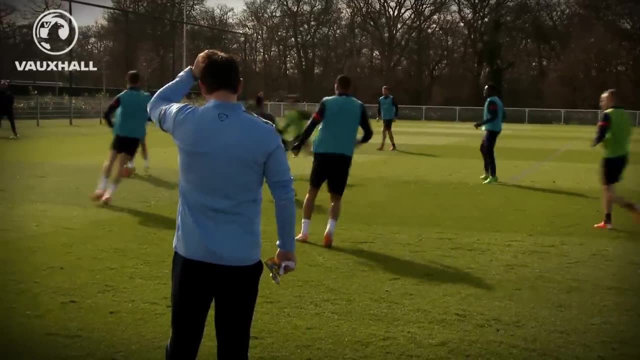 but certainly the importance of the players that they're playing against, the shape of the opposition, the strengths. If there's individual players that our defenders are playing against or midfield players that have got obvious strengths or weaknesses, we make them aware of them and try and not confuse them too much but give them good information. 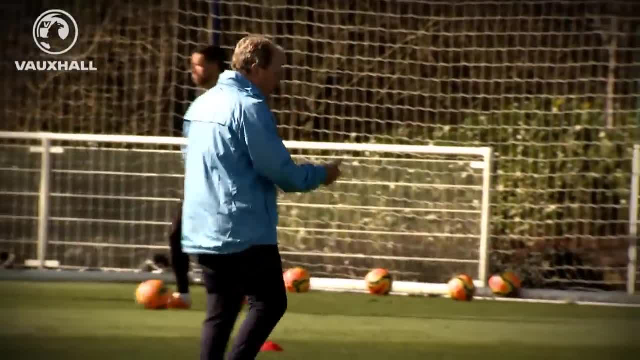 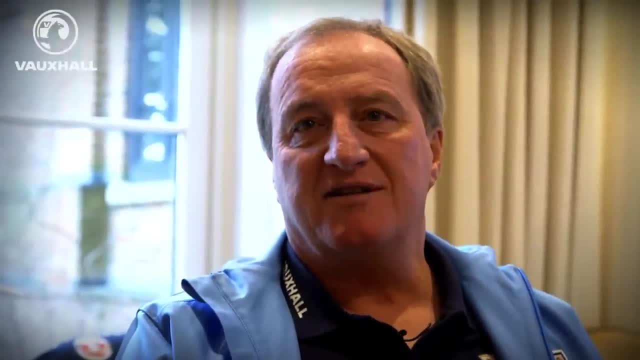 that will enhance their performance and help them win the game. It's a vital tool for us and, compared to before, a lot of it you did on the pitch, you did on trust, that you said this happened during the game, but because there was no, 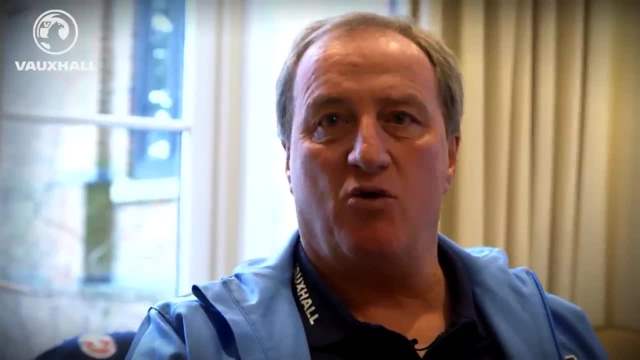 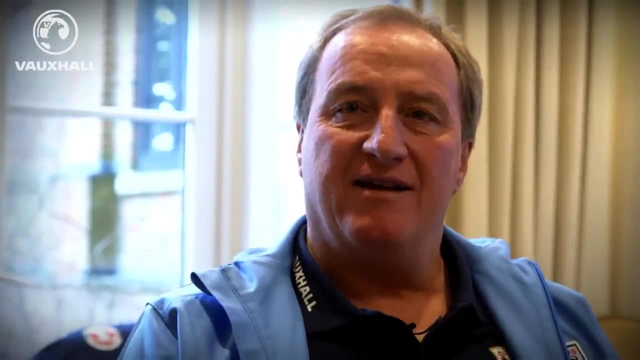 film of it. now we've got the evidence to say this is why this happened. Sometimes it can be for the benefit of the players in as much that we were wrong, but most of the time we're right when we think the players are out of position and we can bring them in and 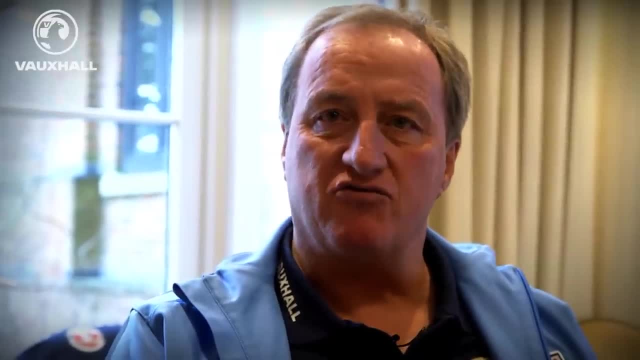 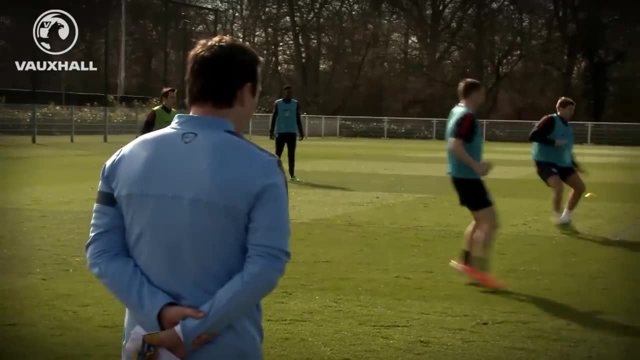 just say: listen, you need to be around a little bit- four or five yards around than you were, or you need to be pushed forward a little bit more, and there's the video evidence to help us to explain it to them. I think simple instructions are the key. 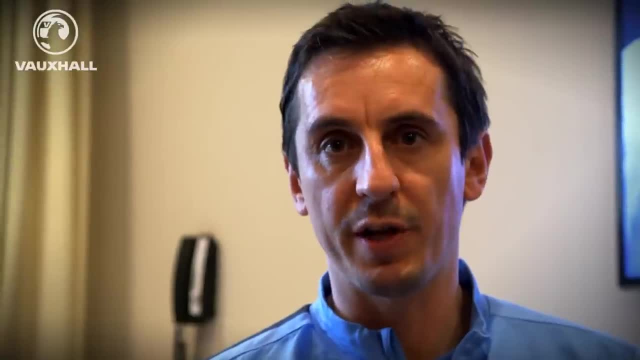 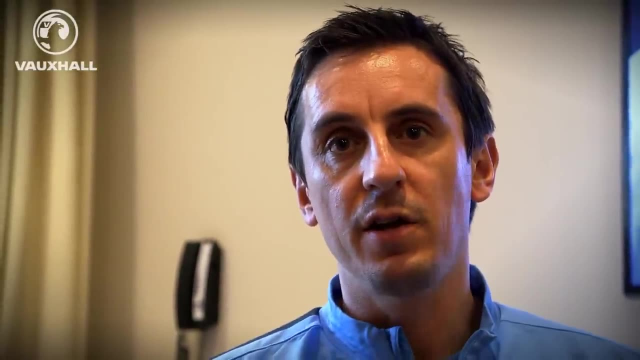 I think definitely, particularly around the opposition. if you're showing an opponent that's going to do something time and time again, you really will, particularly the intelligence of the players at this level that you're dealing with. they do take the information they want. 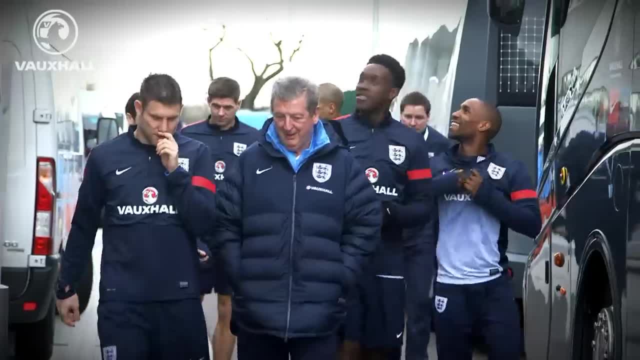 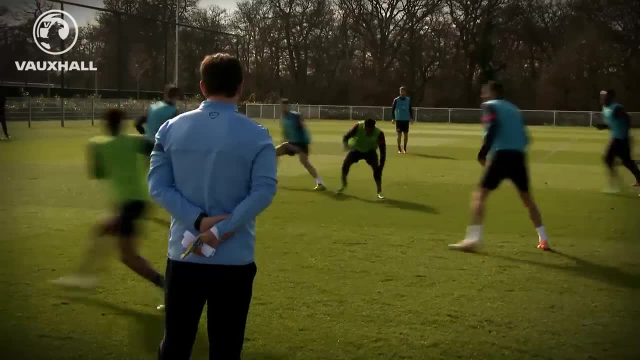 the information they want to be prepared when they go out onto the pitch, and I think that's always as a player. it doesn't change now and hear what we're doing- that you want to try and make sure that the players have got a picture of what's going to happen in. 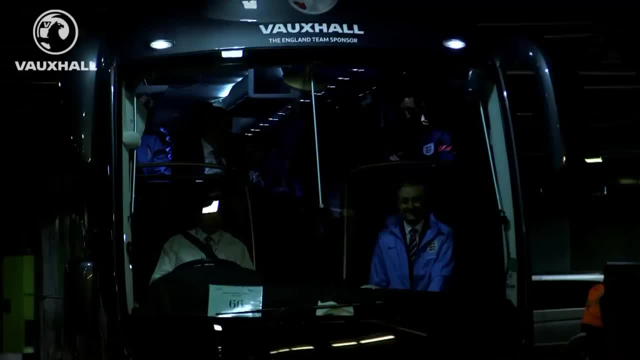 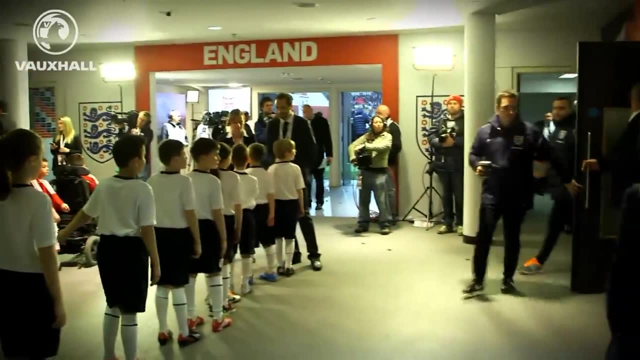 the game in every instance really and prepare them as much as possible. I think it's something that we started probably six months ago in the first half. everybody will know- coaches and managers- that it can get difficult at times to see the bigger picture. 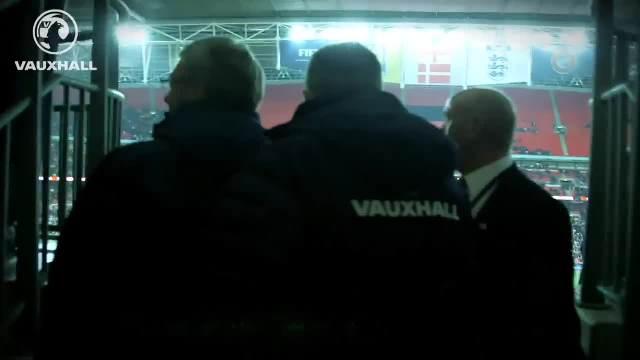 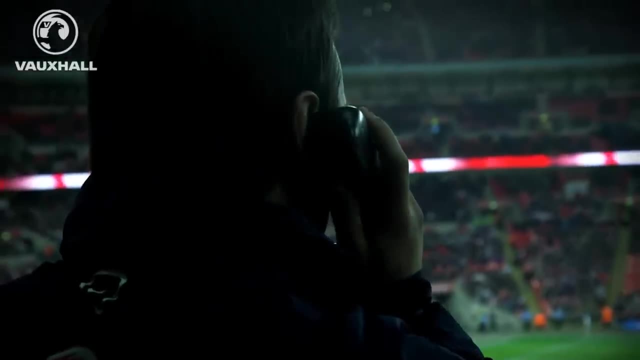 from the touchline. it's just another pair of eyes. obviously, Roy and Ray are on the bench, so the idea that one of us is just sat up there in the higher position maybe see different things and a different sort of perspective. it's just something that when 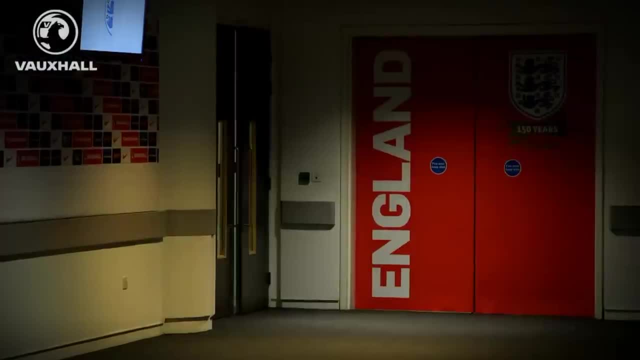 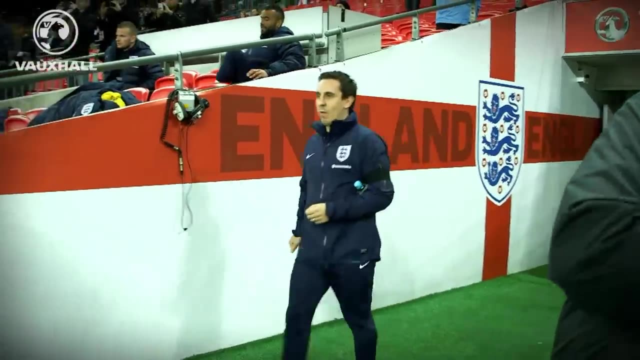 we come in at half-time we can sort of, you know, have a look at it and see what's going on. We can sort of chat between each other about what we've seen from our different areas and different viewpoints, if you like, and obviously in the second half I do go down onto the bench. 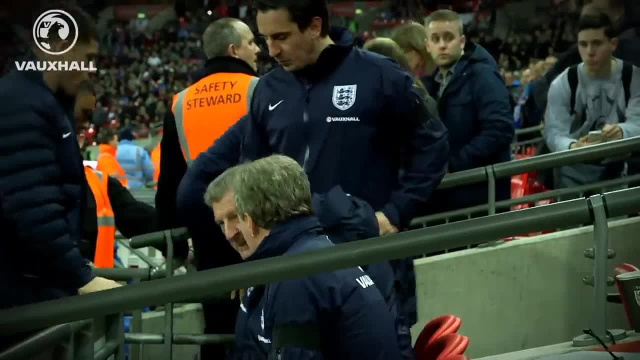 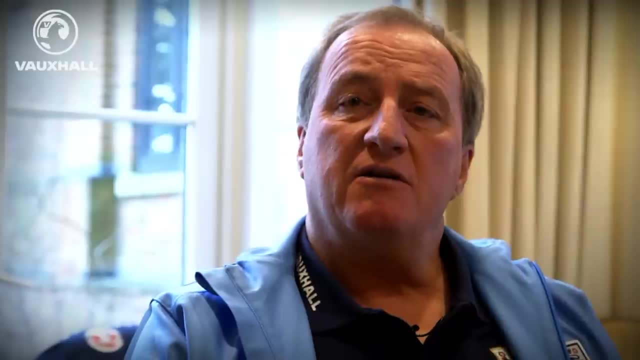 but the first half I do spend up there and I think in some ways it sort of helps you see the game better. obviously, By the time that we kick off into the World Cup we'll know everything we need to know about the opposition, all three teams that we'll be playing at group level, and also we'll 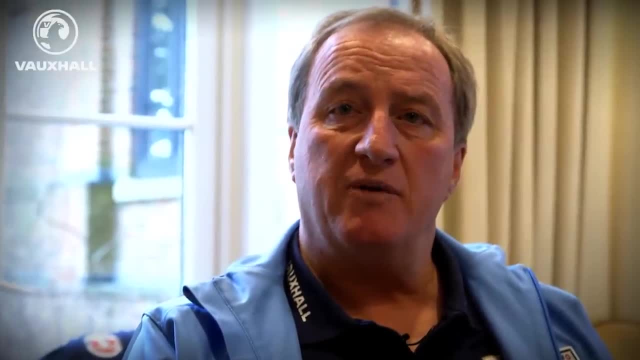 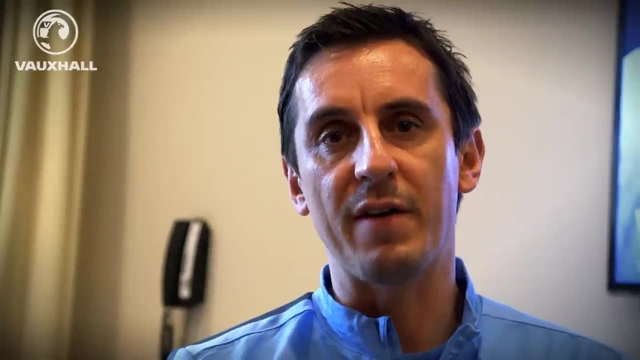 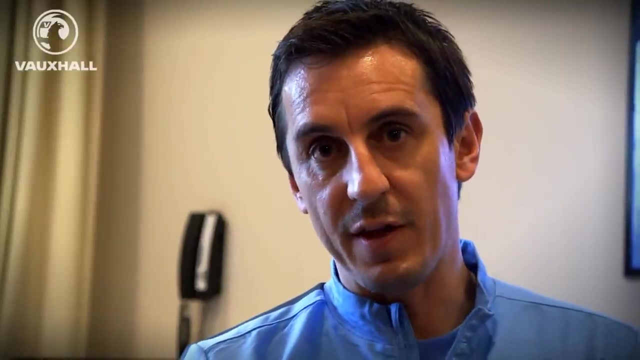 be looking at possible future opponents. that will all be covered. It's critical that obviously building, particularly when you go into a World Cup, you're talking about sort of four or five matches that we'll watch intensely and you see patterns develop of the opposition, strengths and weaknesses. that's the main thing. and then what is it?